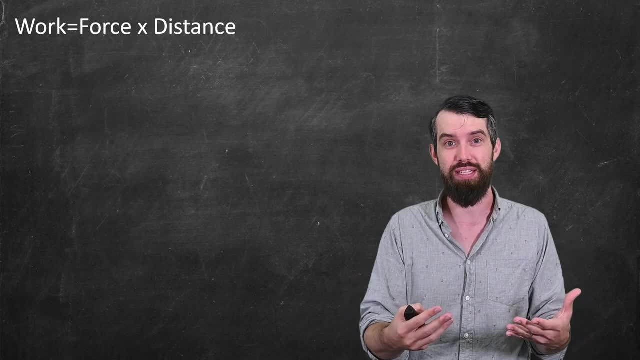 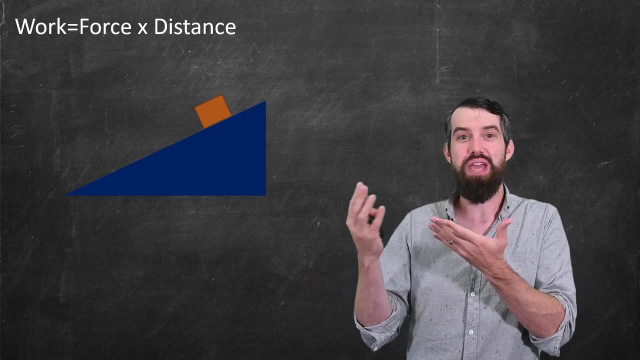 A sort of an elementary way of thinking about what the contract of work is. If you apply a lot of force for a long distance, you've done a lot of work. The standard example of this was an inclined plane. We have a block, The plane is assumed to be frictionless and the block is going to be sliding down the 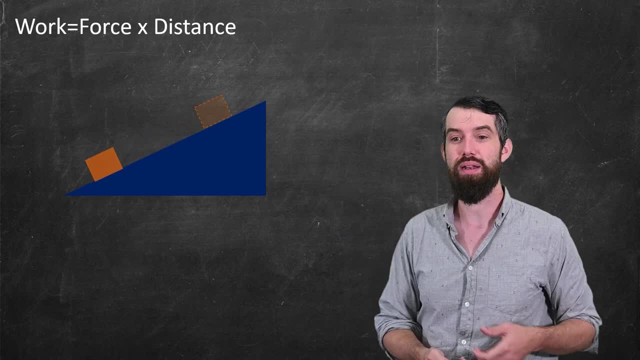 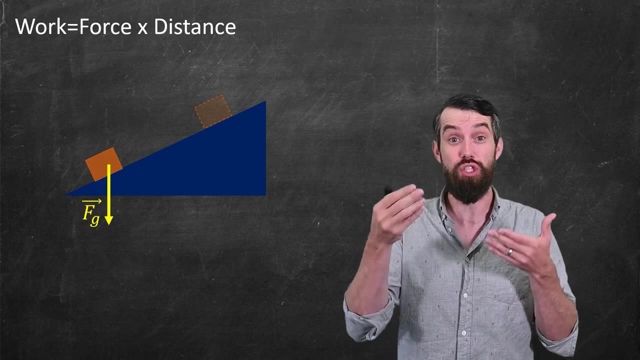 plane under the force of gravity, It might move well, a little bit like this. So if we analyze what's going on, we're going to see that the force of gravity is going to be less than the force of gravity. So what's going on here? there's a force of gravity on that block. that points straight down. But you can. 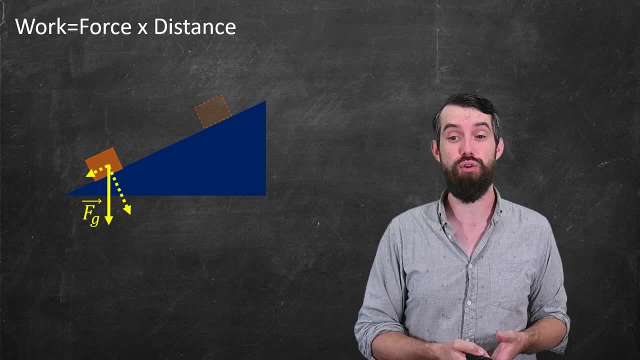 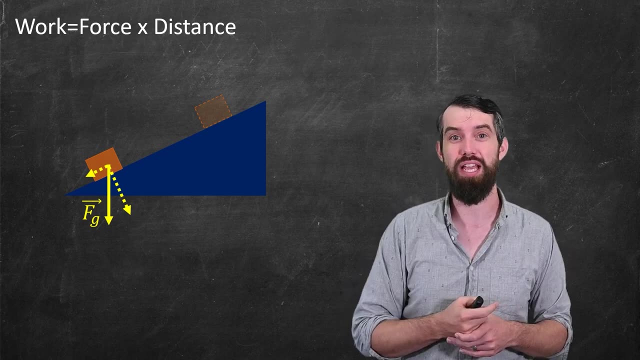 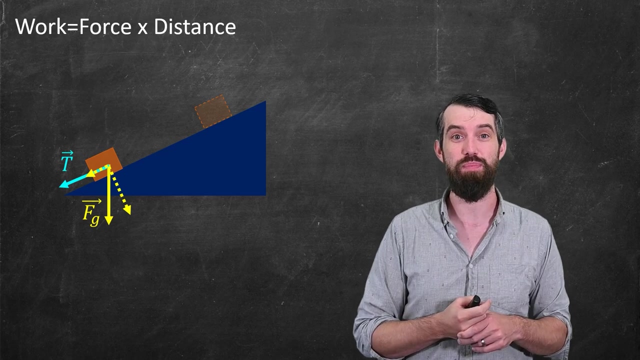 decompose that force of gravity into two different directions: A proportion that is normal to the inclined plane and a portion which is tangential to the inclined plane. Indeed, I'm also going to add a vector, which I'll call t, and this is just showing what is the direction of that inclined 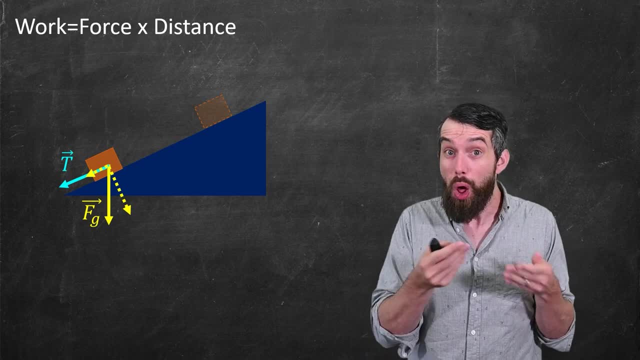 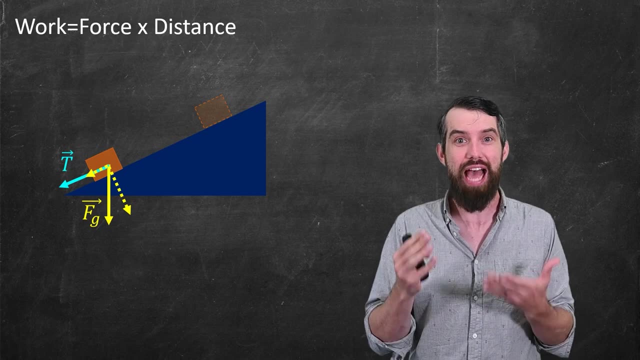 plane. So because the block moved along that inclined plane, the proportion of the force of gravity that was normal is irrelevant. There's no work that's being done in that direction. All of the work that was done was the proportion that was moving in the tangential direction. 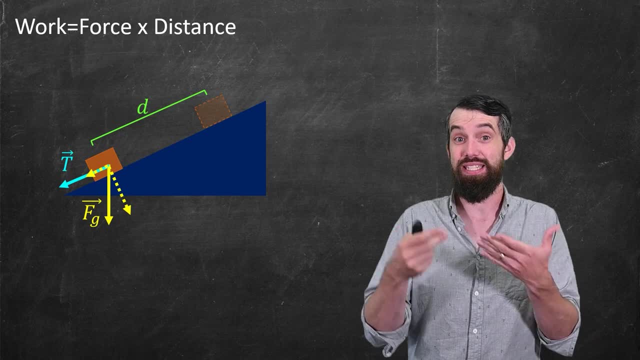 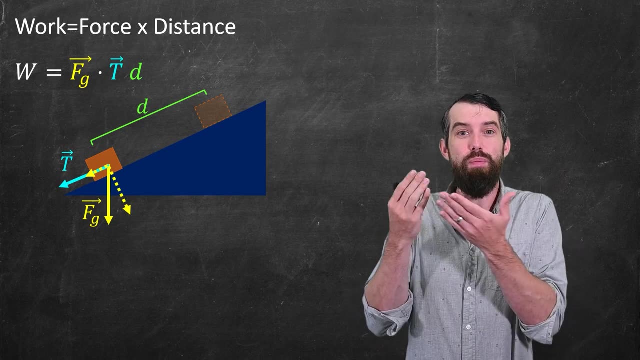 So how much work is actually being done? Well, if we say that there is a distance d between where the block started and where the block ended up, then what we can talk about is the dot product. This is the proportion of the force of gravity in that tangential direction. That's the force. 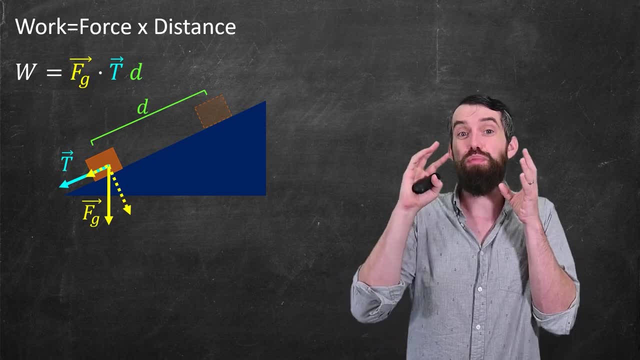 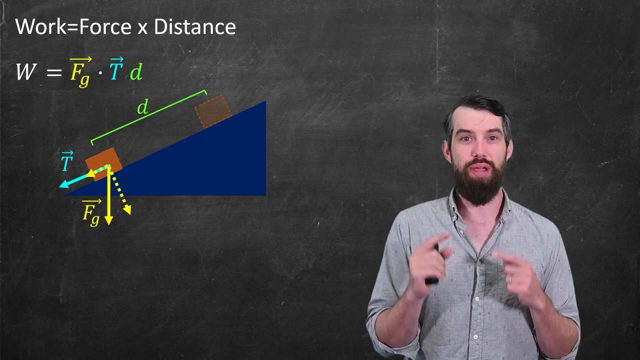 that we're interested in. It's not the entire force of gravity, just the proportion of the force of gravity, And that's what a dot product captures. And then you multiply that by the distance d Okay. so pay attention to the fact that our work here was defined to be a force dotted with the. 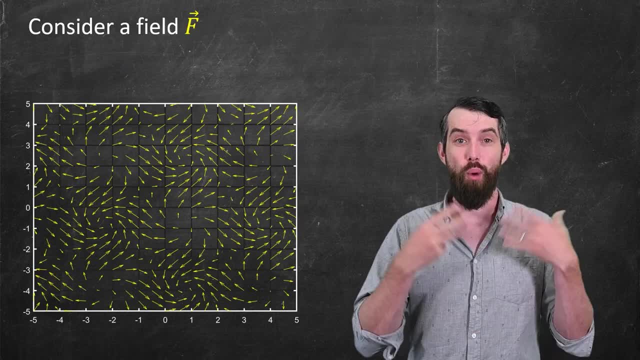 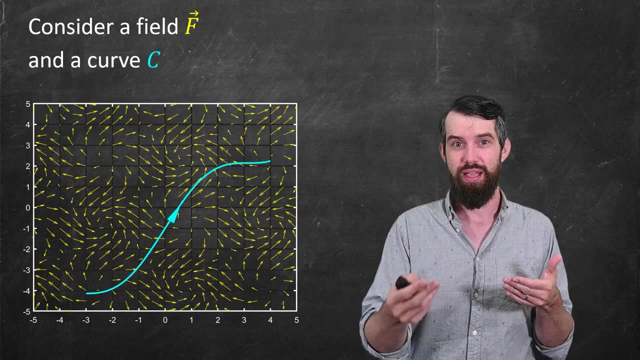 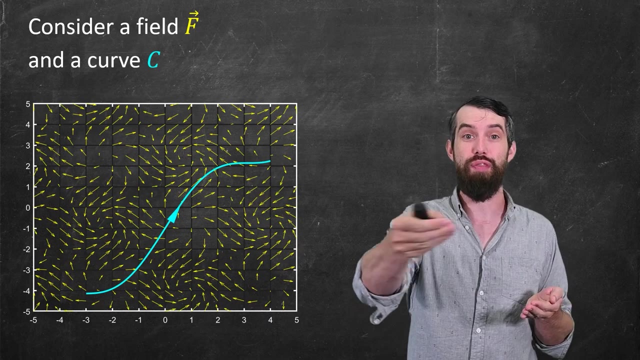 tangential. And let's zoom back out to our more complicated situation, where I have some field And then I have a curve that is going to be going through that field And then the question is, what is the work done by that field if I move some particle along that curve? And, as we just saw, 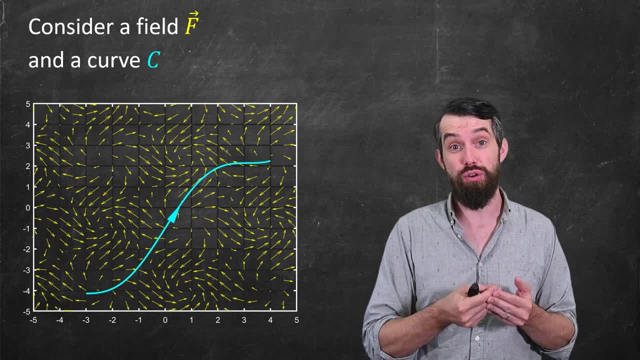 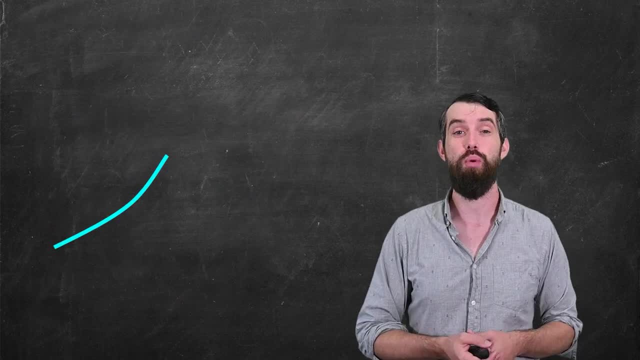 the answer to how much work done is going to depend on the degree to which this curve is going tangential to the field. So let me zoom in on a little portion of the curve and analyze what's going on here. So if I take some spot and I'm going to measure a little unit of ds, I'm going 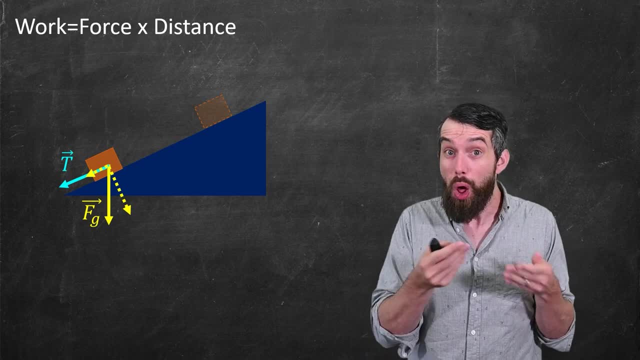 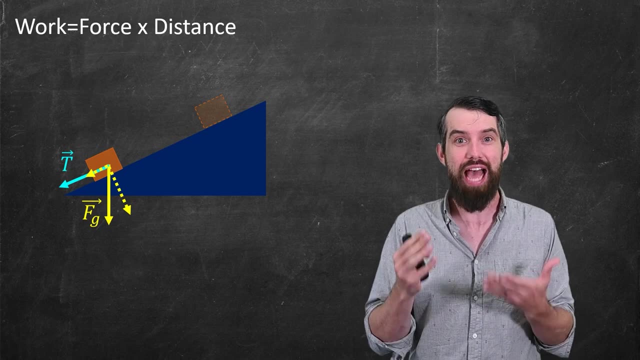 plane. So because the block moved along that inclined plane, the proportion of the force of gravity that was normal is irrelevant. There's no work that's being done in that direction. All of the work that was done was the proportion that was moving in the tangential direction. 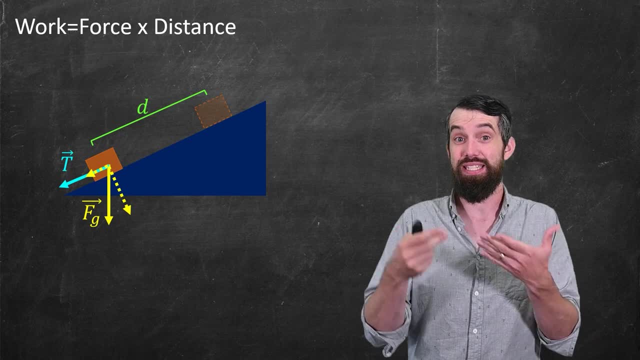 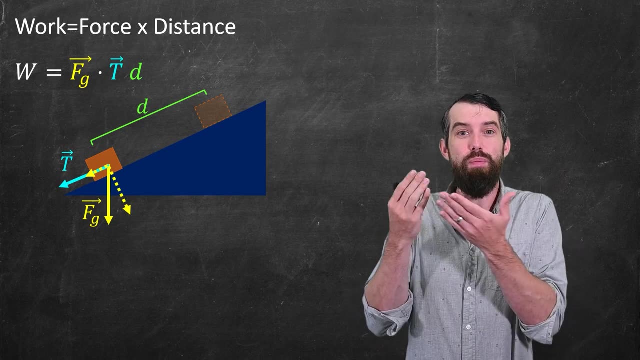 So how much work is actually being done? Well, if we say that there is a distance d between where the block started and where the block ended up, then what we can talk about is the dot product. This is the proportion of the force of gravity in that tangential direction. That's the force. 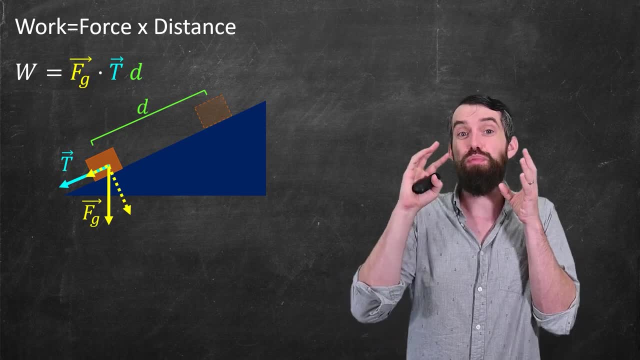 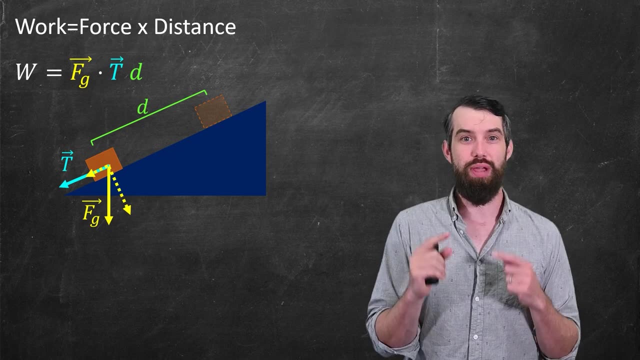 that we're interested in. It's not the entire force of gravity, just the proportion of the force of gravity. This is the proportion of the force in the tangential direction, and that's what a dot product captures. Then you multiply that by the distance, d. Okay. so pay attention to the fact that our 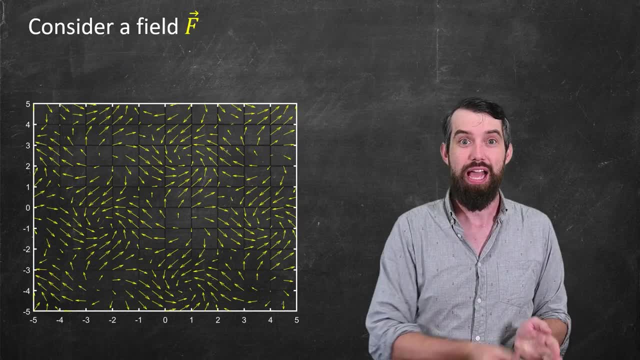 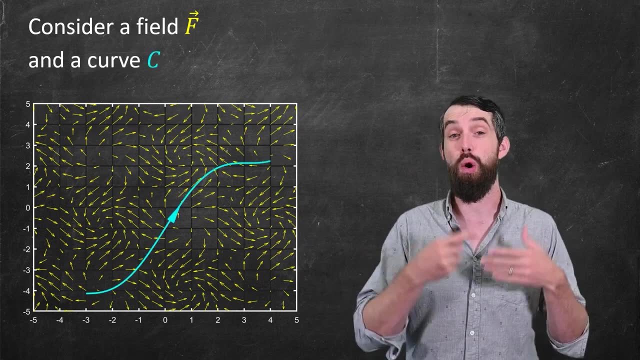 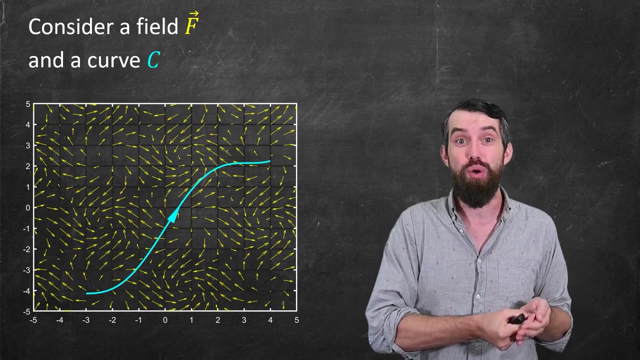 work here was defined to be a force dotted with the tangential. and let's zoom back out to our more complicated situation where I have some field and then I have a curve that is going to be going through that field. Then the question is: what is the work done by that field if I move some particle? 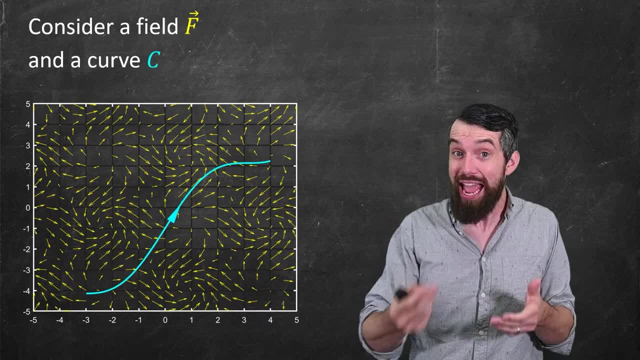 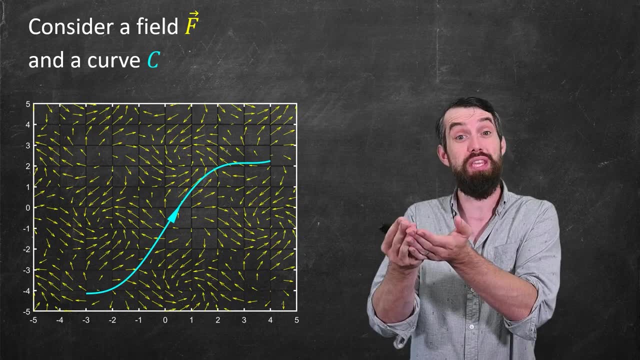 along that curve. As we just saw, the force is a force of gravity, Then I have some field and then a curve of gravity saw. the answer to how much work done is going to depend on the degree to which this curve is going tangential to the field. So let me zoom in on a little portion of the curve and 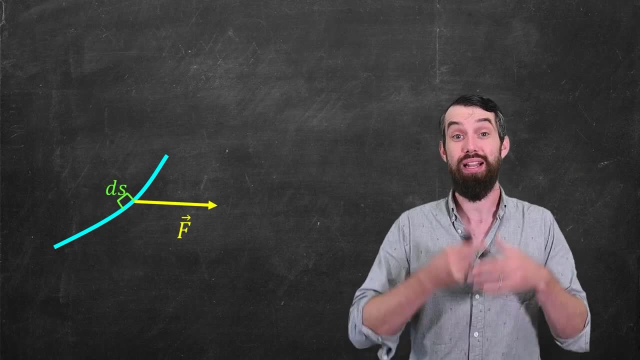 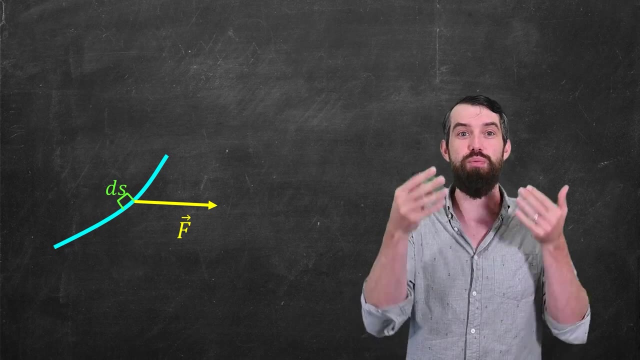 analyze what's going on here. So if I take some spot and I'm going to measure a little unit of ds, I'm going to imagine that I'm just moving some small amount along the curve, a little change in arc length, we call it ds, And then I'm going to say, well, in that, 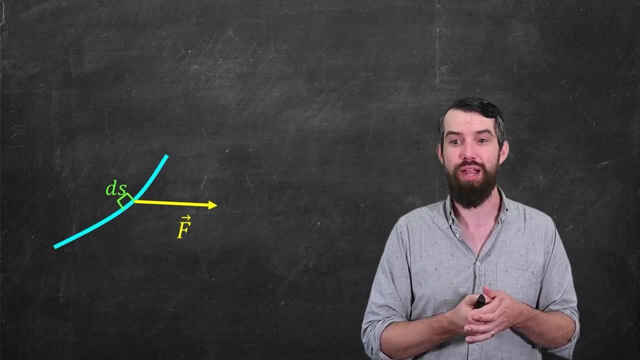 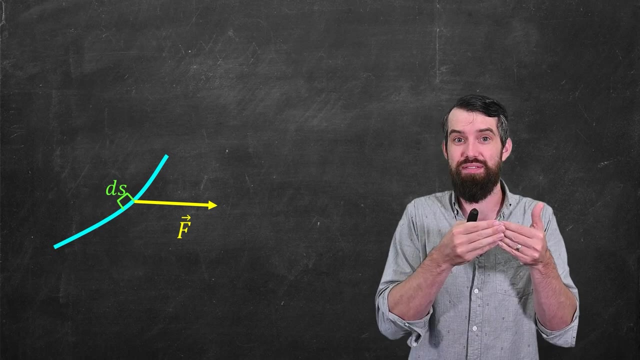 small little region. I'm going to have some vector field, then it's going to point in some direction, so I'll put that vector for the f. And then if I'm interested in what is the work done by this little movement of length ds, I also have to ask: well, what? 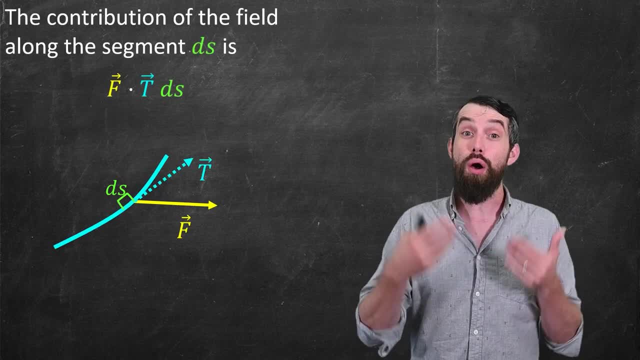 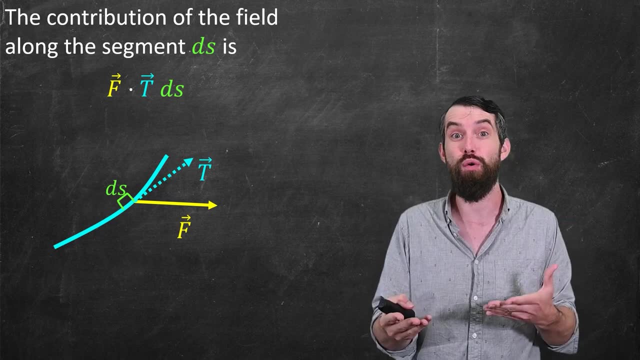 is the tangential component. So then the contribution of the field along that little segment ds is just given by the f dot t, that's the proportion of the force in the t direction times this little ds. If I'm interpreting this as work, then I would say the work done. 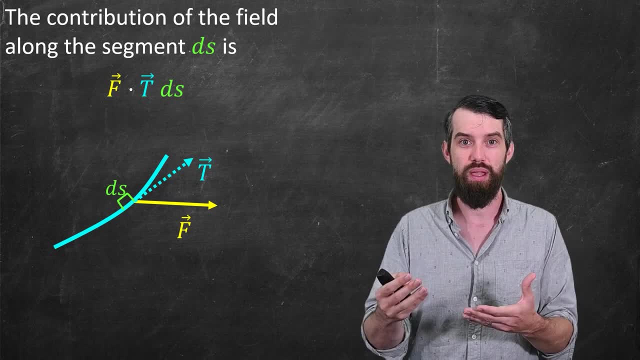 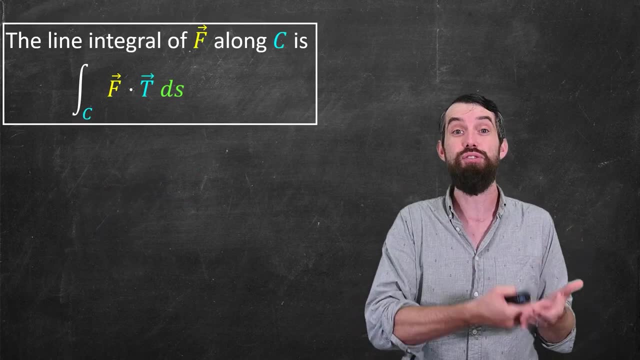 from moving that little ds is this: f dot t. Subtitles by the Amaraorg community. Finally, I had a much bigger curve and so if I want to add everything up, I'm just going to integrate it. I just do the line integral of a vector field f, along the curve c. it's. 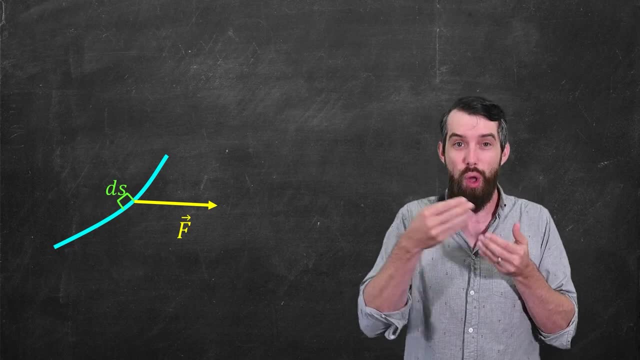 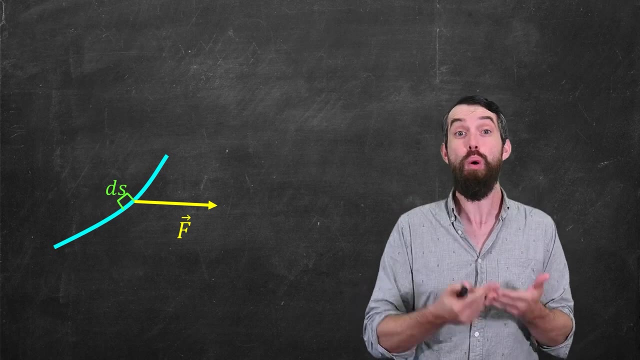 to imagine that I'm just moving some small amount along the curve. a little change in arc length, we call it ds, And then I'm going to say, well, in that small little region I'm going to have some vector field. Then it's going to point in some direction, So I'll put that vector for the f. 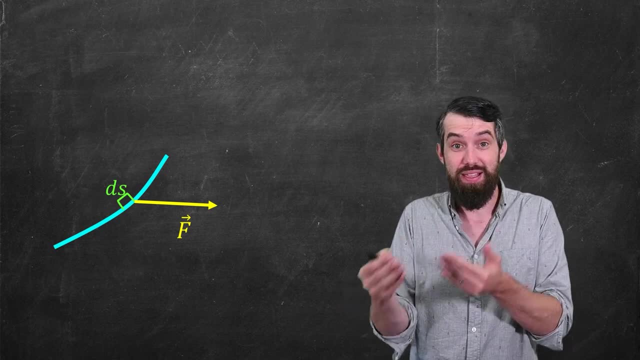 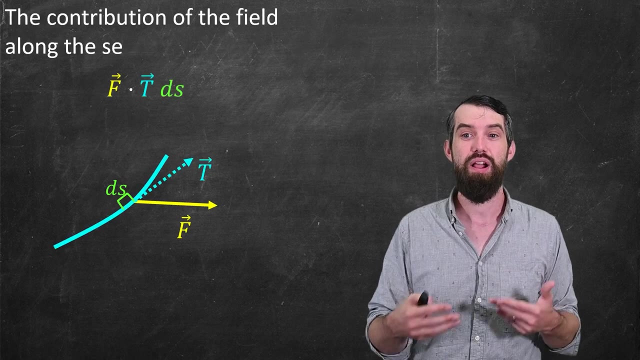 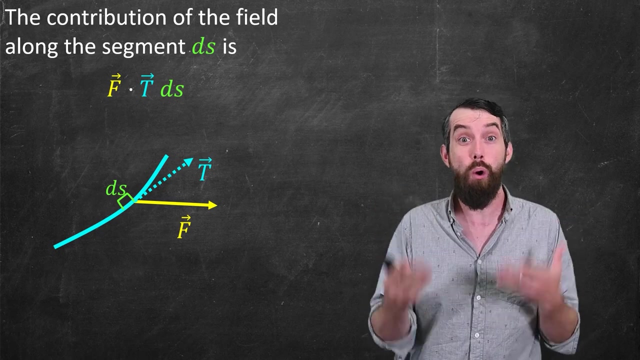 And then, if I'm interested in what is the work done by this little movement of length, ds, I also have to ask: well, what is the tangential component? So then, the contribution of the field along that little segment ds, is just given by the f dot t, that's the proportion of the force. 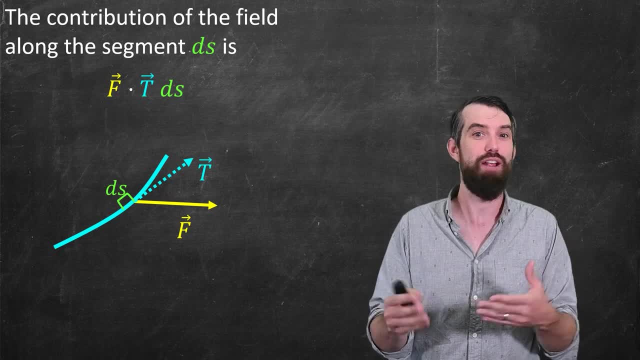 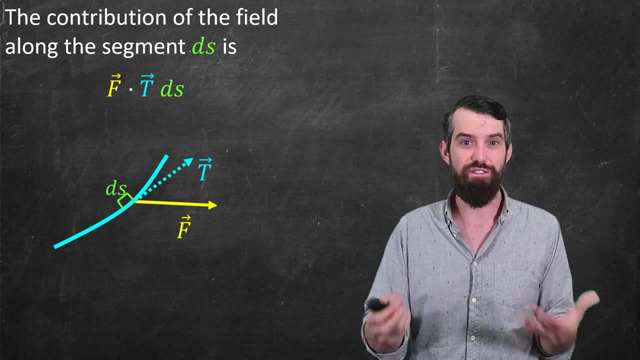 in the t direction times this little ds. If I'm interpreting this as work, then I would say the work done from moving that little ds is this: f dot t ds. Finally, this is a much bigger curve, and so if I want to add everything up, I'm just going to integrate it. 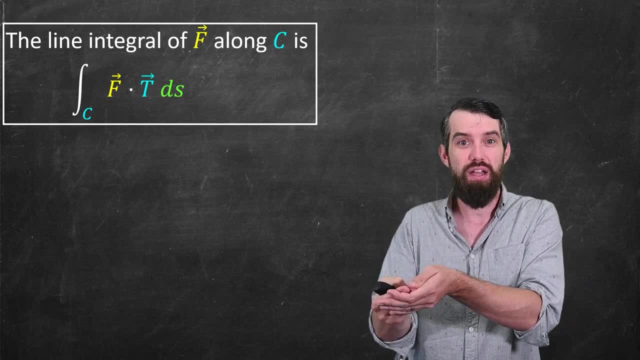 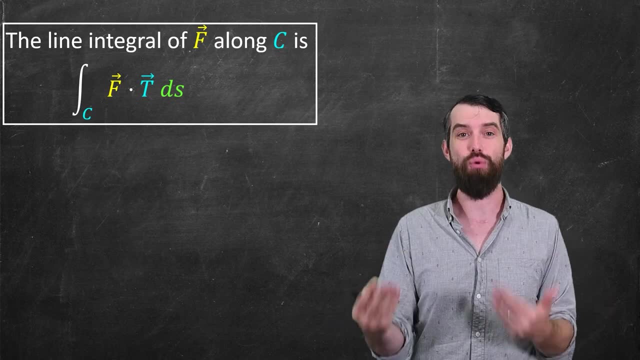 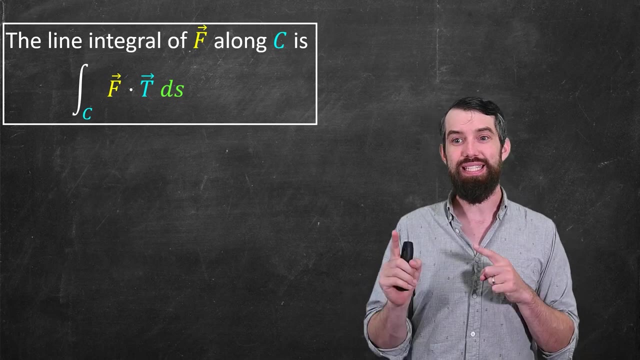 I just do. the line integral of a vector field f along curve c is just given by this integral over c, the same line integral we've seen before. it's just that the integrand is the f, dot, t and then integrated with respect to ds. So this formula is exactly like the line integral formula we've. 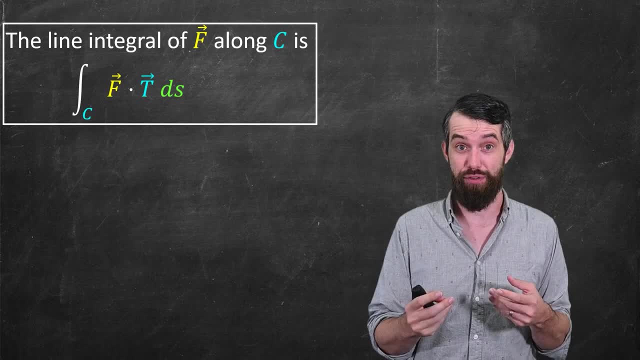 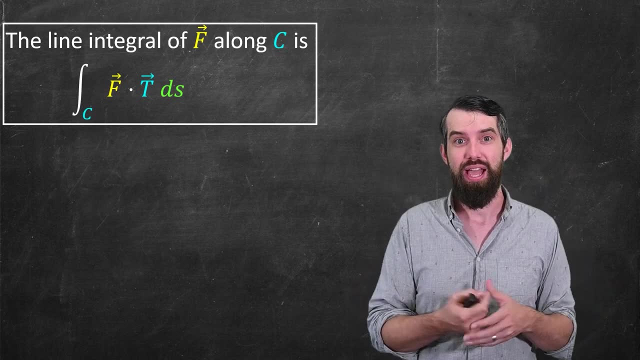 seen before. indeed, it's defined in the exact same way, it's just the integrand is different. It's not an arbitrary function, which is what we've seen before. the integrand is the specific thing. it's trying to capture the influence of the field along the curve, and so the integrand is. 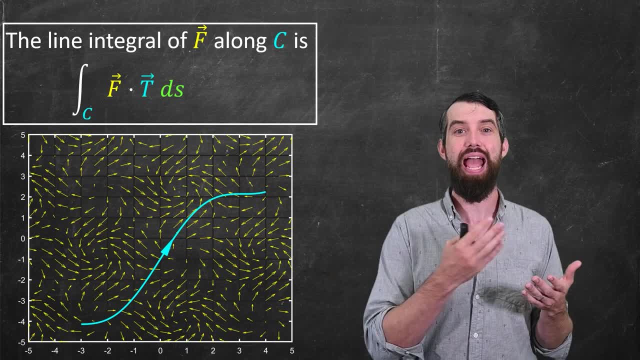 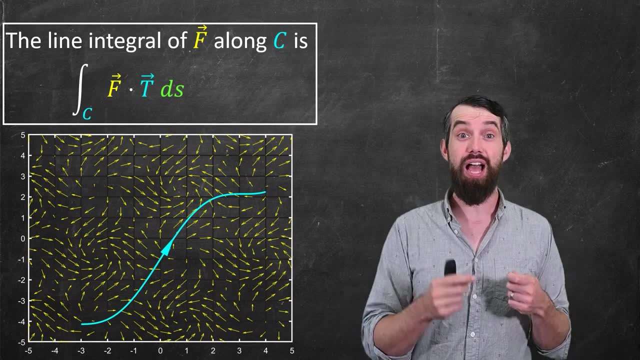 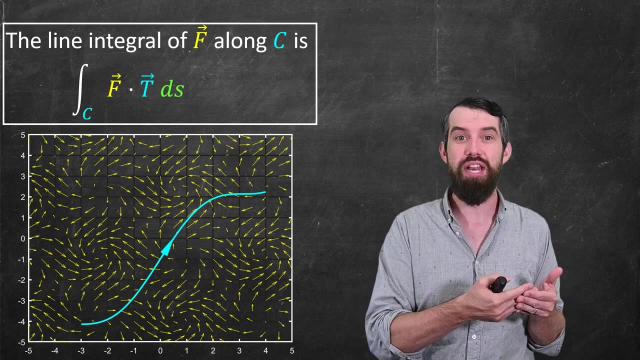 this f dot t And so putting the picture back up, we have an answer to the work done. if you move the particle along this curve, in this particular field- And indeed I've been talking about work so far in this video- that specific physics concept, but indeed the concept of a line integral, 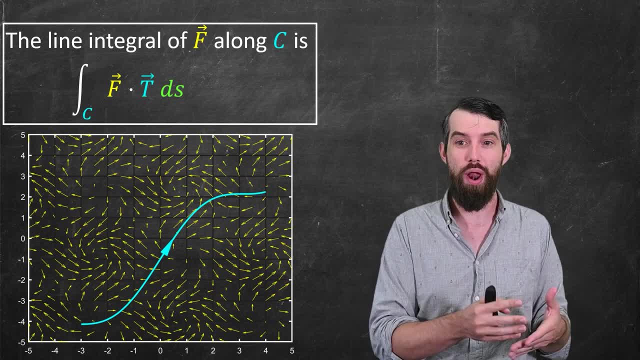 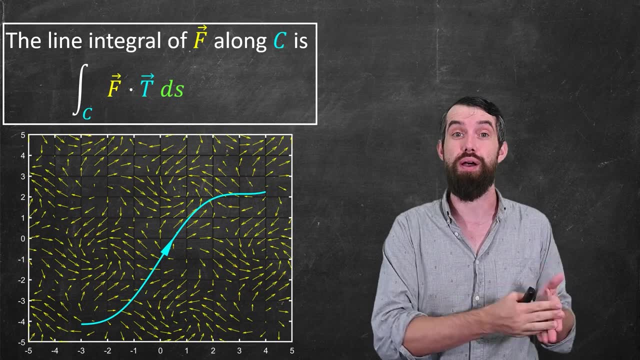 a long-term curve is something that applies in many different scenarios. work is just one of them, so this definition applies broadly. This is a definition we can understand, because we previously understood the concept of a line integral. But the question now is: how do we? 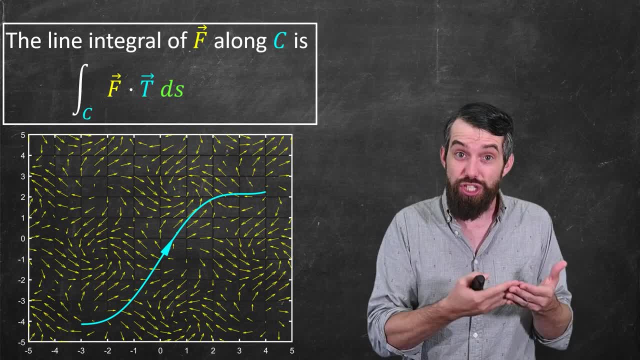 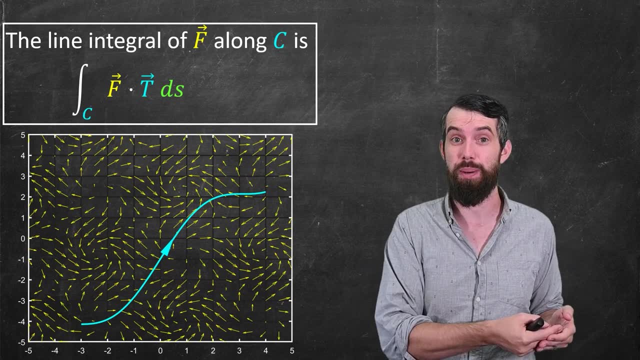 compute it And, as we've seen before when it comes to computations, we want to see how can I parameterize a curve explicitly and then rewrite this formula in terms of that parameterization. Okay, so let's give some labels. I'm going to say I have a parameterized curve, The curve is on some. 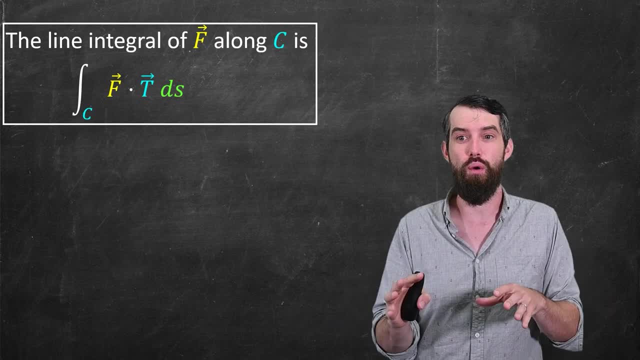 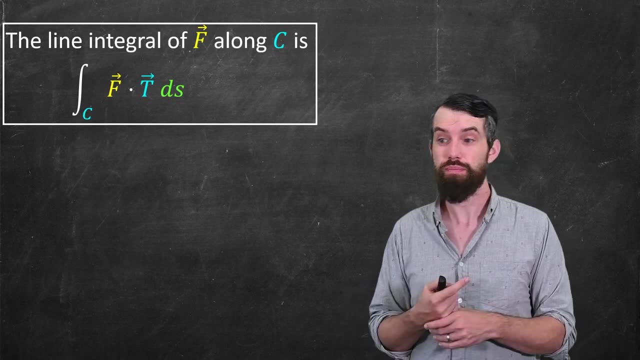 just given by this integral over c, the same line integral we've seen before. it's just that the integrand is the f dot t and then integrated with respect to ds. So this formula is exactly like the line integral formula we've seen before. indeed it's defined in: 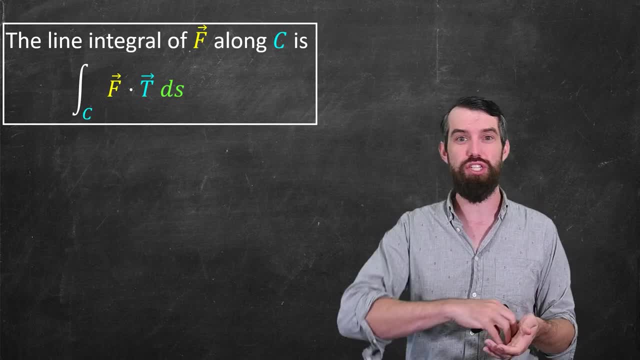 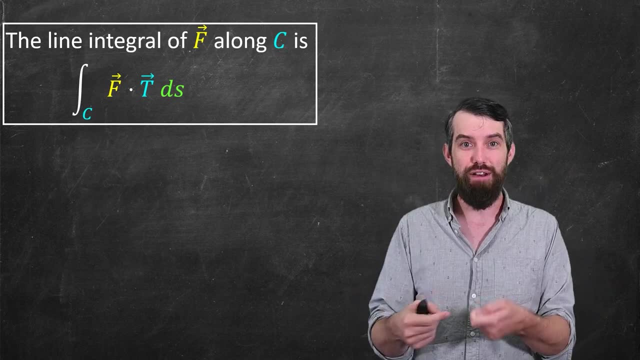 the exact same way. it's just the integrand. The integrand is not just an arbitrary function, which is what we've seen before. the integrand is this specific thing: it's trying to capture the influence of the field along the curve. 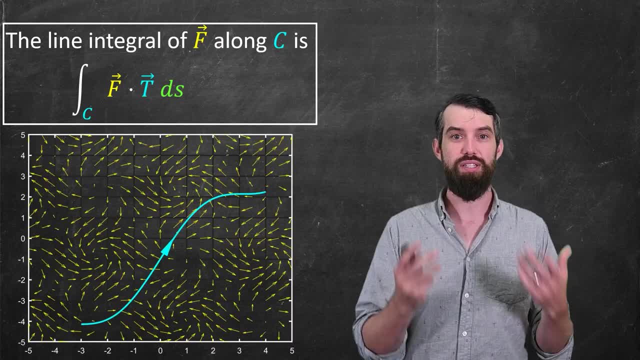 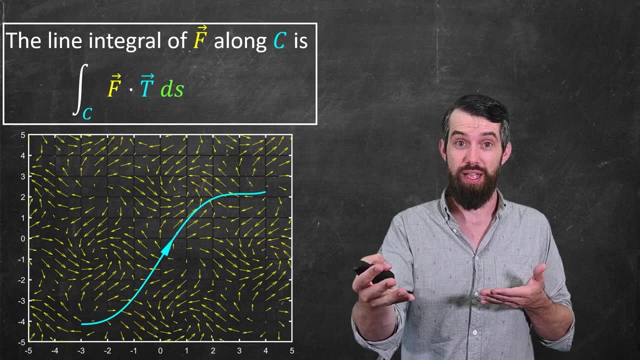 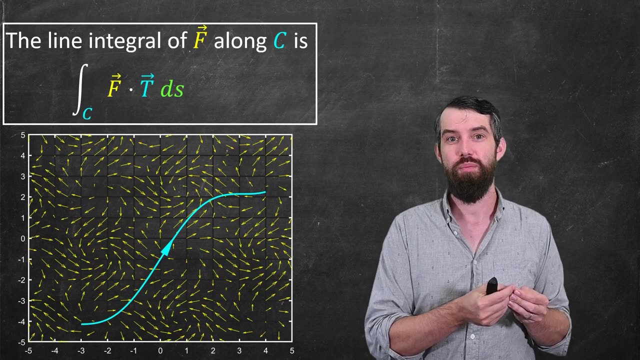 and so the integrand is this: f dot t, And so, putting the picture back up, we have an answer to the work done if you move the particle along this curve in this particular field- And indeed I've been talking about work so far in this video- that specific physics concept, 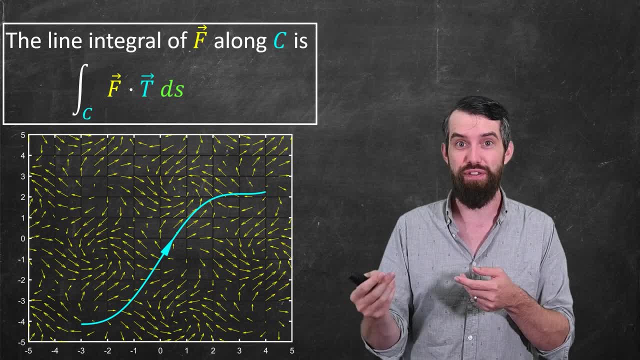 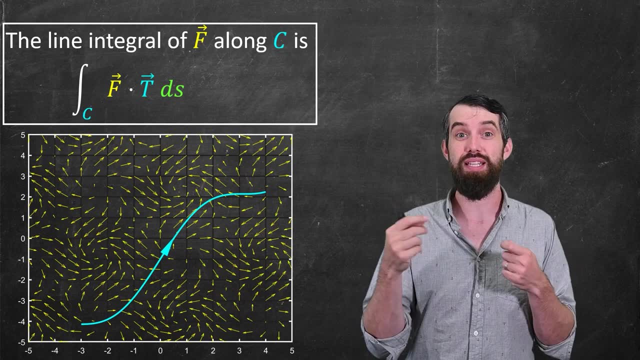 but indeed the concept of work is not the same as the work done in this particular field. Subtitles by the Amaraorg community. The concept of a line integral of a vector field along some curve is something that applies in many different scenarios. work is just one of them, so this definition applies broadly. 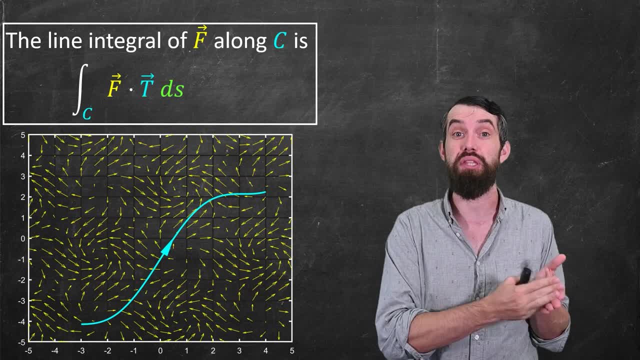 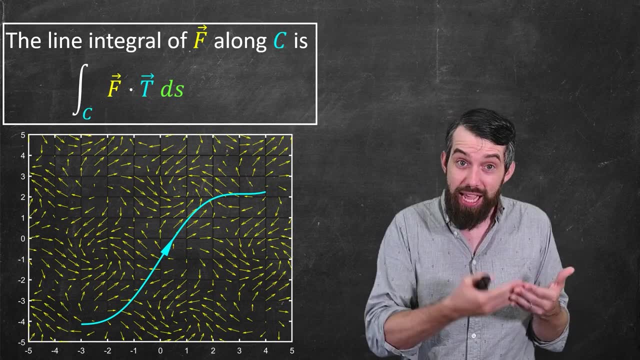 This is a definition we can understand, because we previously understood the concept of a line integral. But the question now is: how do we compute it? And, as we've seen before when it comes to computations, we want to see. how can I parameterize a curve explicitly? 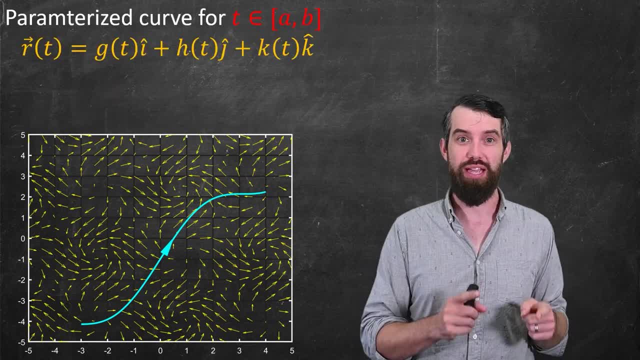 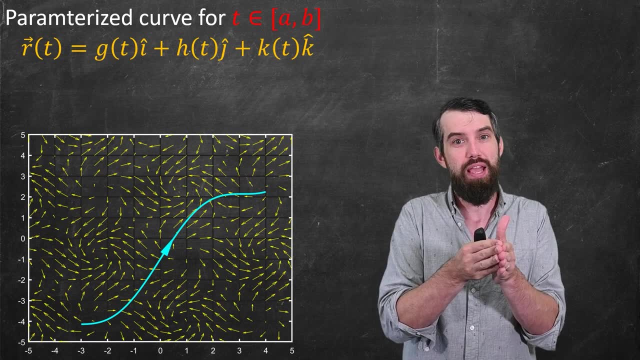 and then rewrite this formula in terms of that parameterization. Okay, so let's give some labels. I'm going to say I have a parameterization and then I have a price curve. The curve is on some interval of t- t between a and b, and then 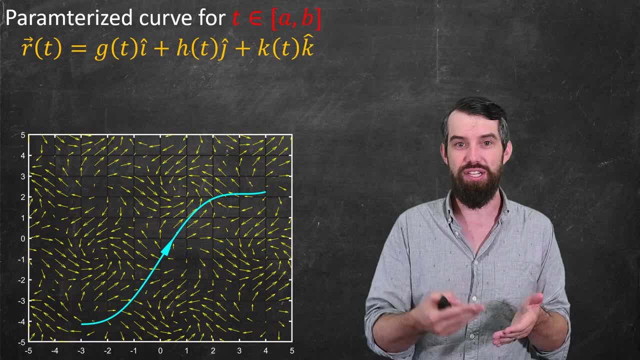 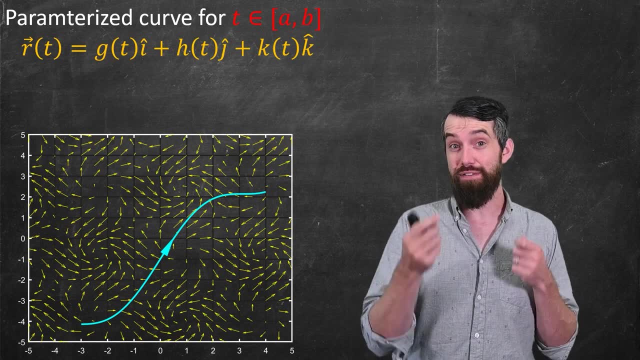 the curve is going to be a g of t in the i-hat, an h of t in the j-hat and a k of t in the k-hat. The way I think about this is: the vector r is a vector that goes from the origin. 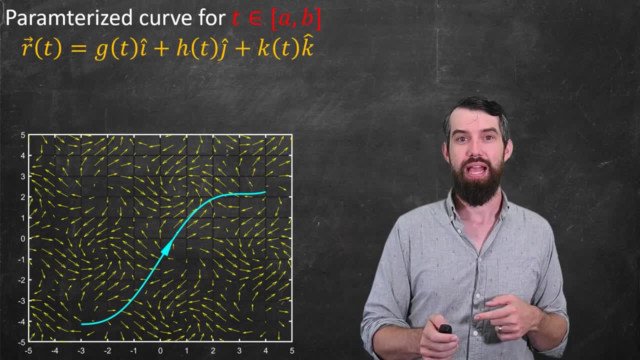 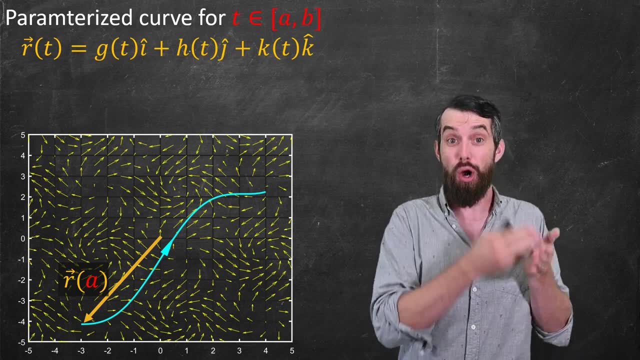 out to the curve. So the origin is in the center of this plot- then the r of a- so that's sort of the first component on my interval of t from a up to b, points to the start of the curve and then the r of b points to the end of the curve. Note, by the way, the curve. 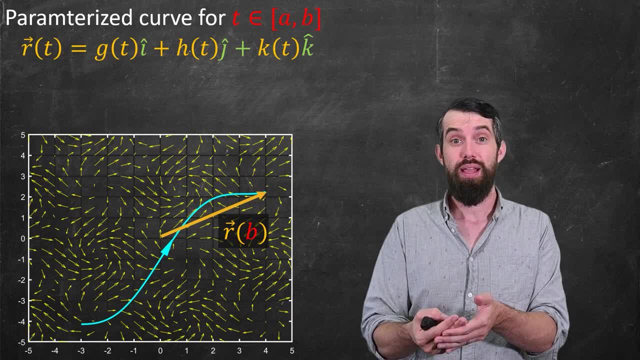 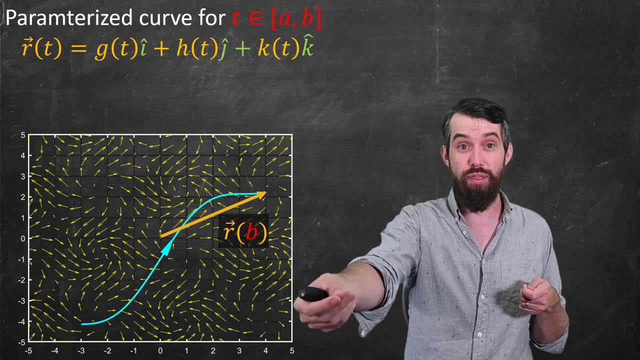 has a little blue arrow here that indicates the direction that it's moving. Indeed, this is going to be very important. When we think about curves, we always want to think about them as starting at one spot and going to another spot. These are sort of directed curves. 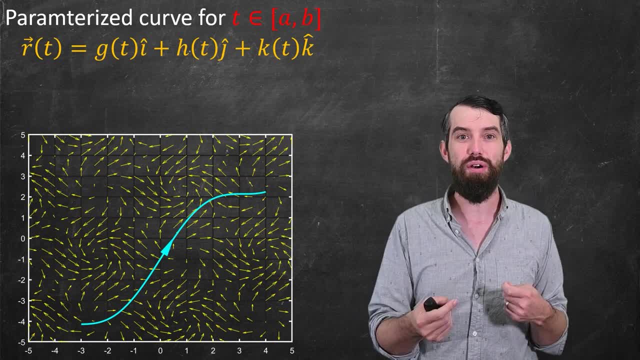 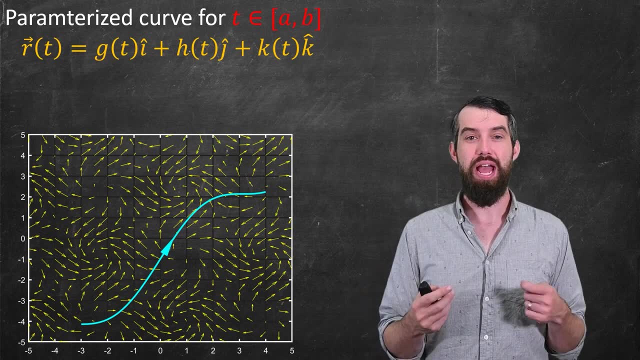 interval of t, t between a and b, and then the curve is going to be a g of t in the i-hat, an h of t in the j-hat and a k of t in the k-hat. The way I think about this is the vector r. 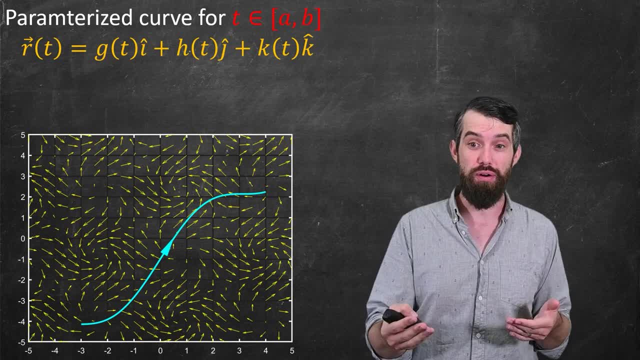 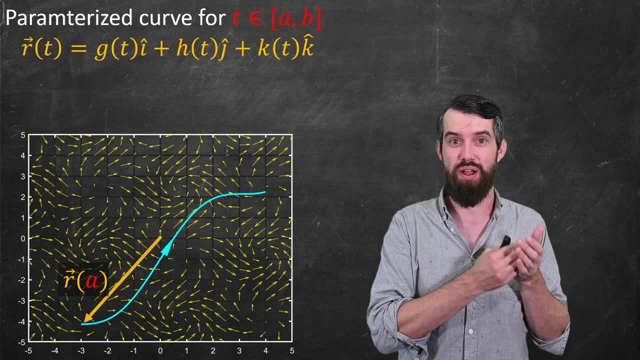 is a vector that goes from the origin out to the curve. So the origin is in the center of this plot, then the r of a, so that's sort of the first component on my interval of t from a up to b points to the start of the curve and then the r of b points to the 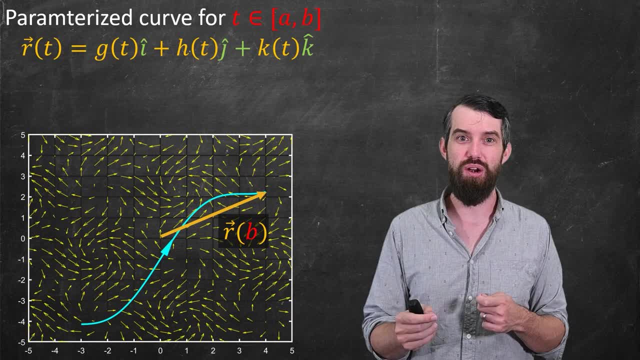 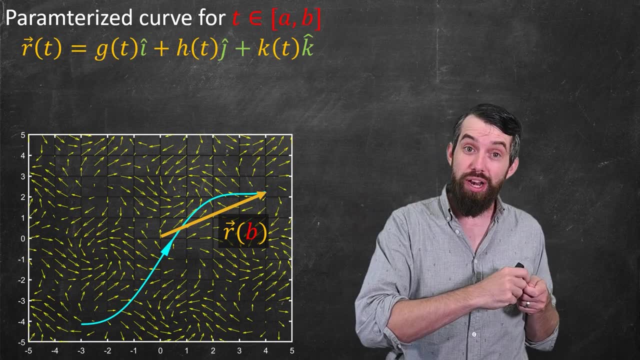 end of the curve. Note, by the way, the curve has a little blue arrow here that indicates the direction that it's moving. Indeed, this is going to be very important. When we think about curves, we always want to think about them as starting at one spot and going to another spot. These are sort 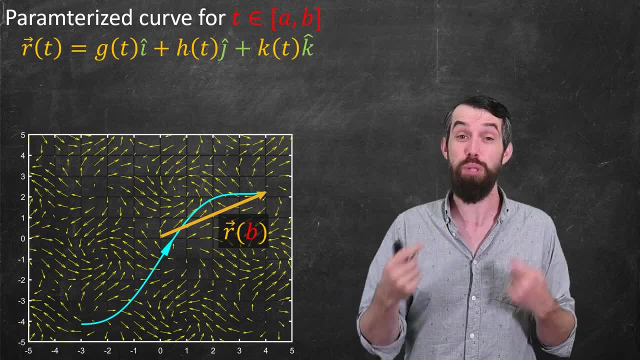 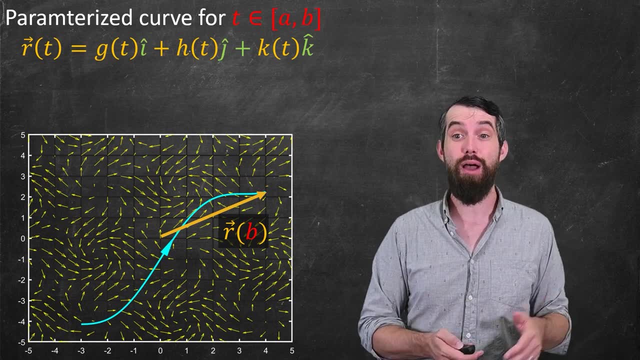 of directed curves. They have a direction that you're traveling and that's implied by this choice of parameterization as well. Okay, so that's the parameterization for the curve. So now I want to go back to the formula I had. There are several changes I can make. Notice how there's the unit. 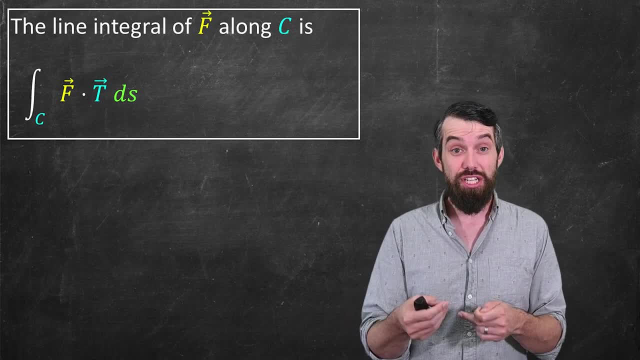 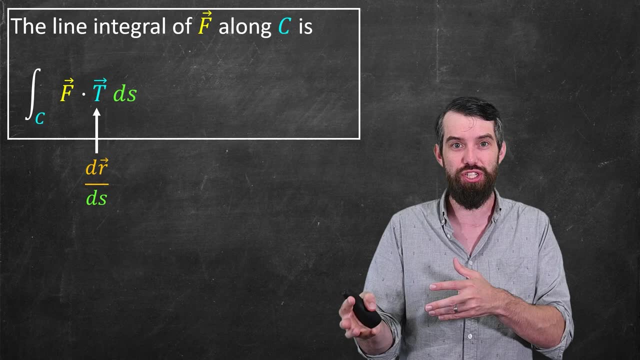 tangent vector t in this formula. Well, a definition of the unit tangent vector t was just that: it was the derivative dr ds. So if you have a specific parameterization you can say: well, how much does that position vector change as you increase arc length? That was a definition. 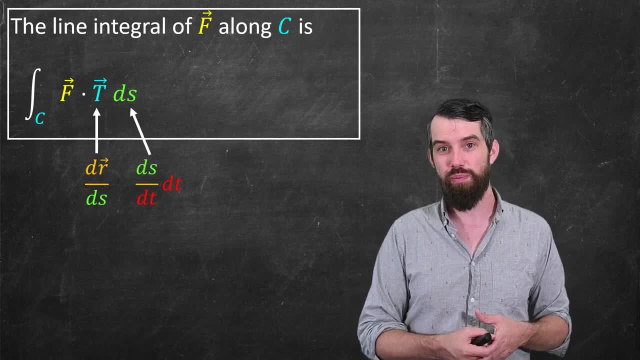 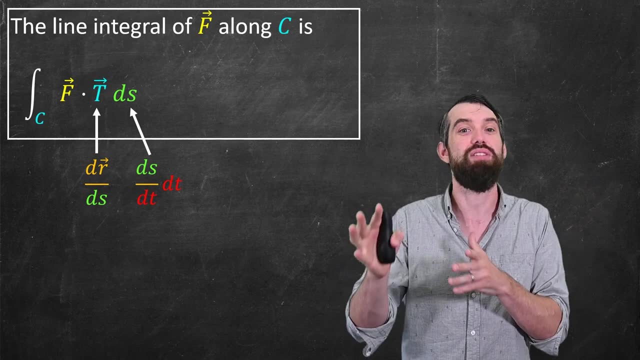 of the unit tangent vector And then just by the chain rule ds, I could replace that with ds, dt, dt. So, again with chain rule, the ds's cancel. I mean they don't cancel exactly, but that's the result of the. 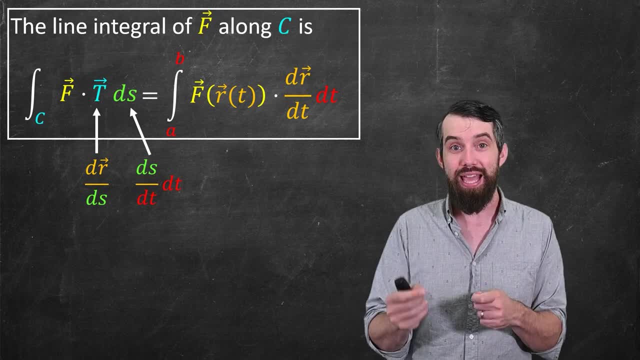 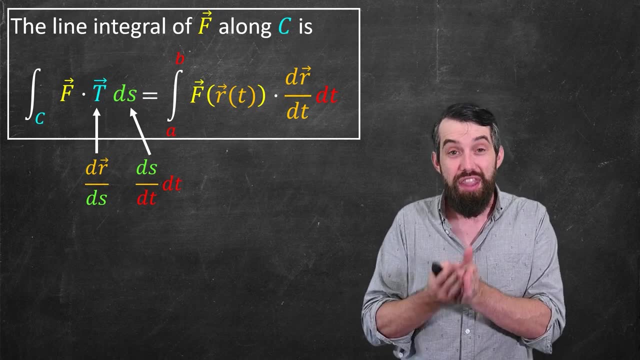 chain rule And, as a result, I can plug this in and what I get is the field just evaluated now along the curve. so f of r of t, And then I multiply it by the derivative dr, dt. That's a dot. 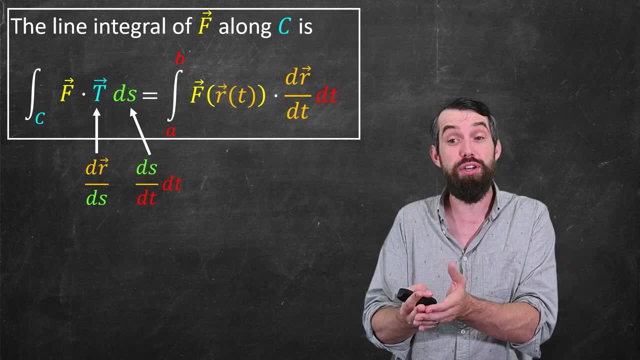 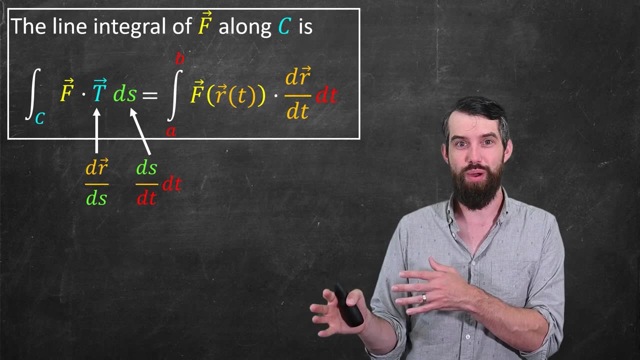 product between this field and this derivative, And then all integrated out with respect to t, and my limits of integration are in t as well. They go from the a up to the b. So well, the left side of this equation is the definition. The right side of this equation tells me: 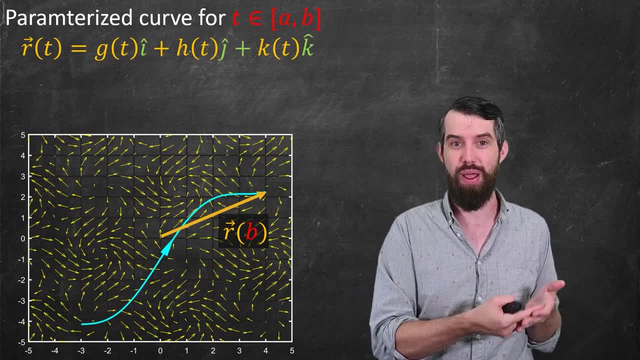 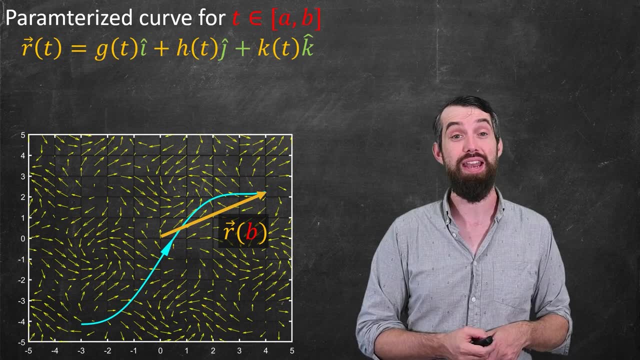 They have a direction that you're traveling And that's implied by this choice of parameterization as well. Okay, so that's the parameterization for the curve. So now I want to go back to the formula I had. There are several changes I can make. Notice how there's the unit tangent vector t in this. 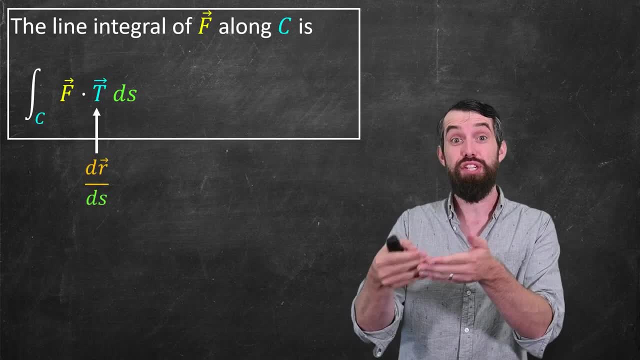 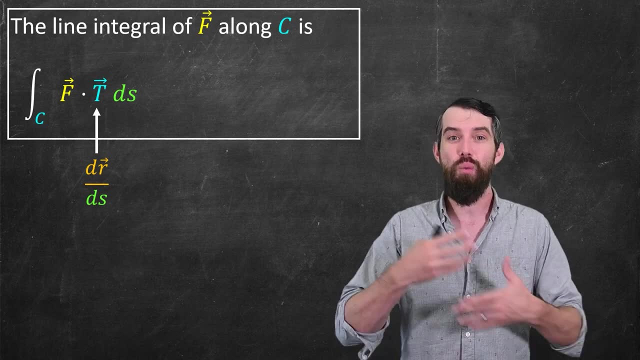 formula. Well, a definition of the unit tangent vector t was just that. it was the derivative dr ds. So if you have a specific parameterization you can say: well, how much does that position vector change as you increase arc length? That was a definition of the unit tangent. 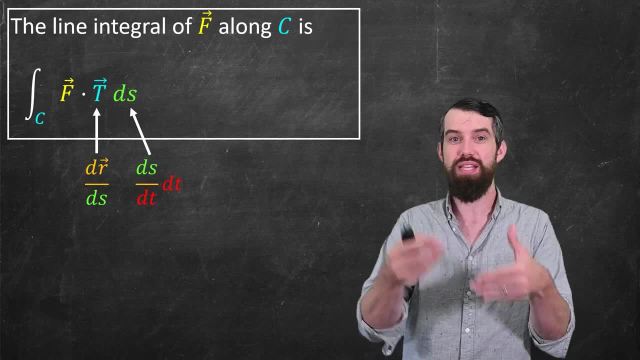 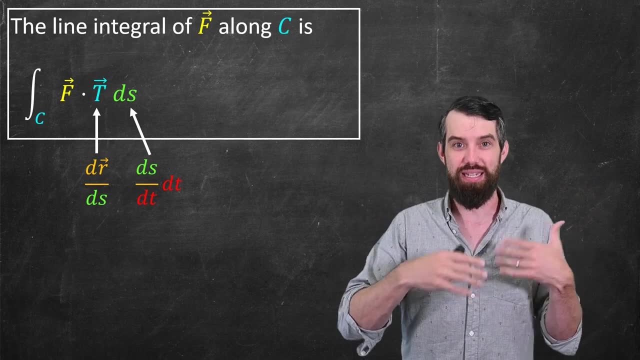 vector, And then just by the chain rule ds, I could replace that with ds, dt, dt. So again with chain rule, the ds is k And if I just simply plug these together I get the result of the chain rule I can plug. 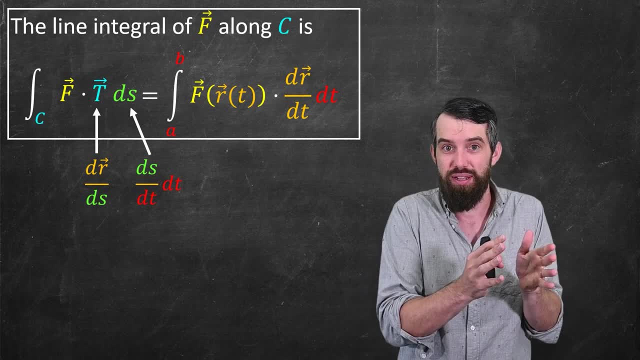 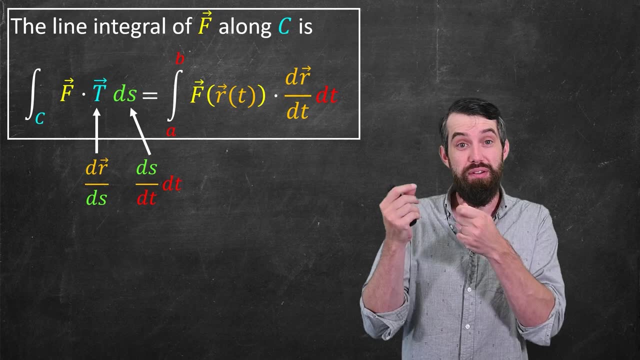 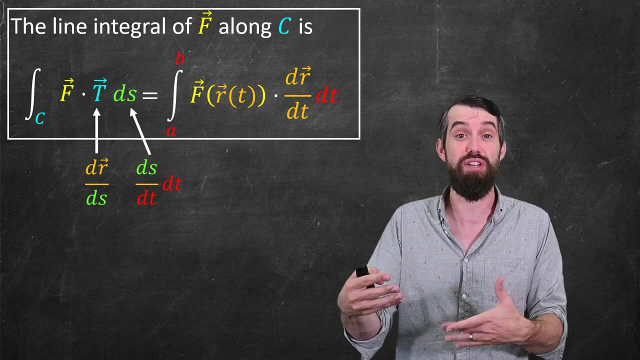 this in and what I get is the field just evaluated now along the curve, so f of r of t, And then I multiply it by the derivative dr, dt, That's a dot product between this field and this derivative, And then I'll integrate it out with respect to t and my limits of 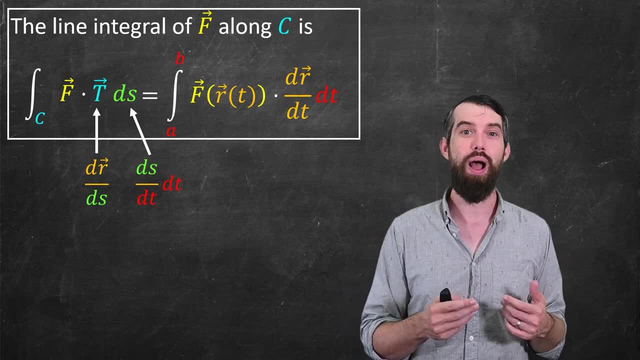 integration r and t as well, that go from the a up to the b. So well, the left side of this equation is the definition. The right side of this equation is the equation. There's a right side of the equation that's the bottom one, and the left side is the left side of. 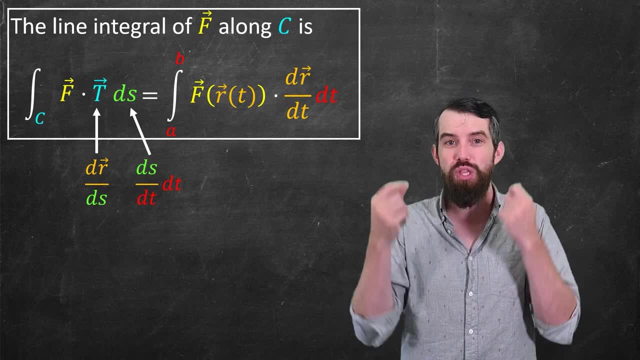 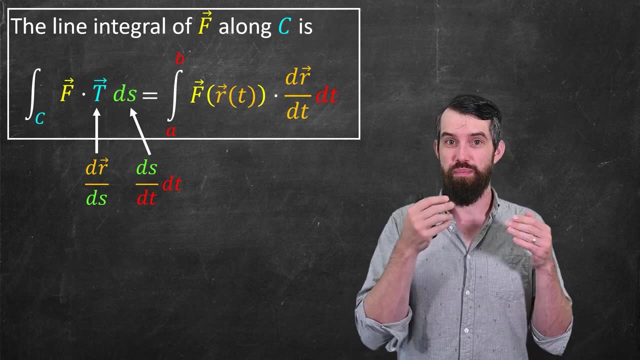 the equation And that's the function of the lóg. So in this equation you can call it, the right side of this equation tells me how I compute it, It gives me an explicit way to compute this And indeed we're going to run through a concrete example: computing a vector field along a curve in. 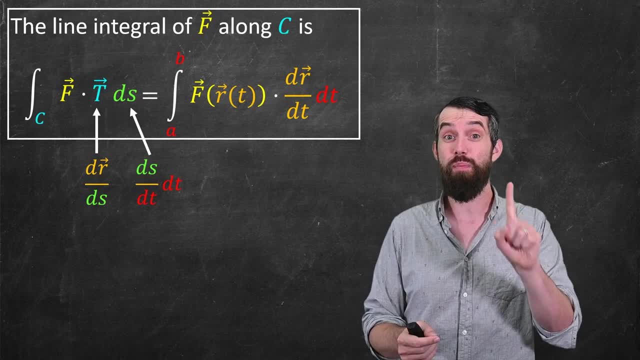 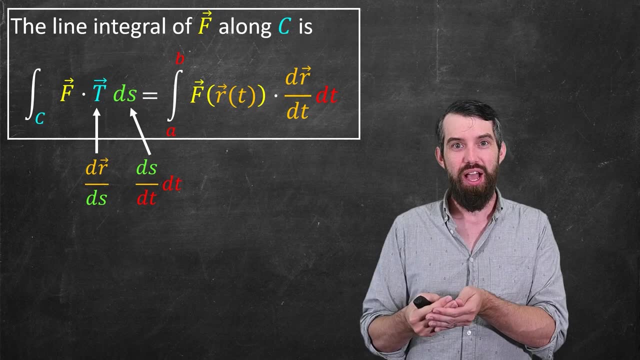 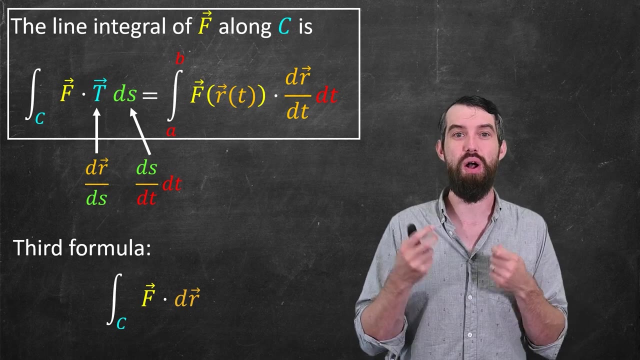 the next video, But before we end I want to show you just one more piece of terminology. It's a third way to think about this. If we have this dr, dt, dt, I can just define a new symbol which is just dr, just to be a shorthand for that. And so my third way of writing this is the integral along. 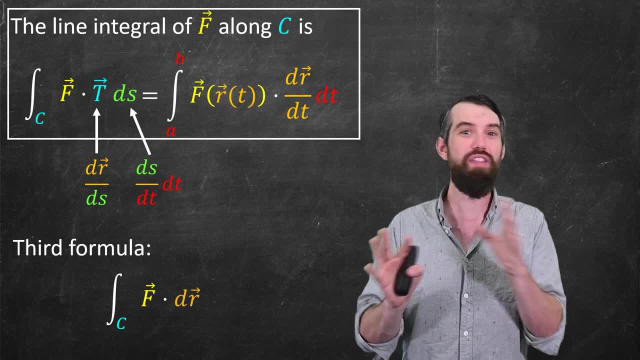 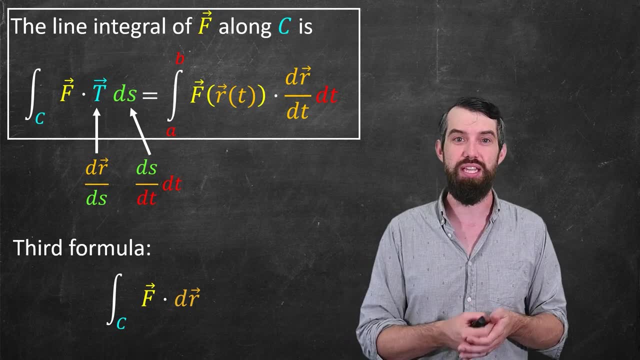 the curve of f dot dr And all of these things are the same, It's just different terminology. So sometimes you'll see a line- integral- written f dot dr. Sometimes you'll see it written f dot t ds. Whenever you want to compute it, though, whenever you actually have an explicit parameterization,